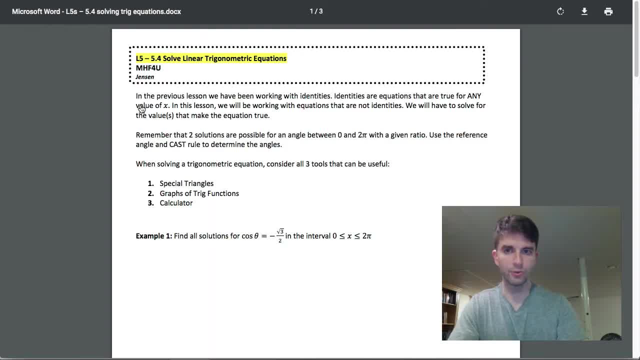 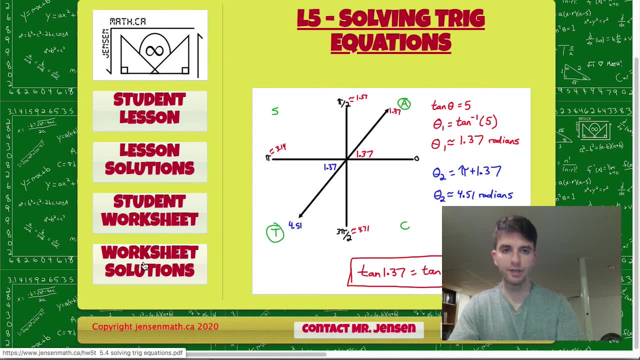 And you can get a blank copy of the lesson there that you can fill out as we go through the video And then, after the video, you can try the practice problems in the student worksheet. And after you try the practice problems you can check your work by looking at this link. 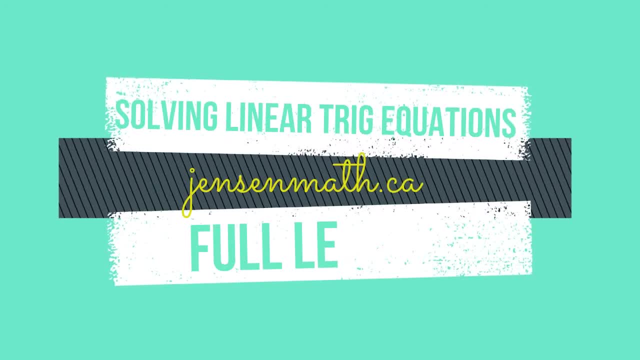 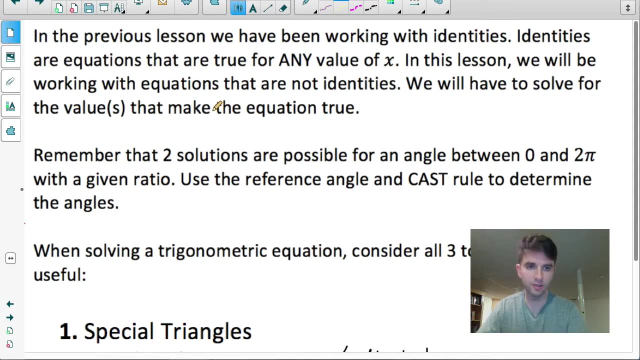 So let's get started. So in this lesson we're going to work through four examples, four equations that need to be solved. Before we do that, let me just orient you in terms of the unit, So the first half of the unit, we've worked with equations that are identities and we worked at proving identities. 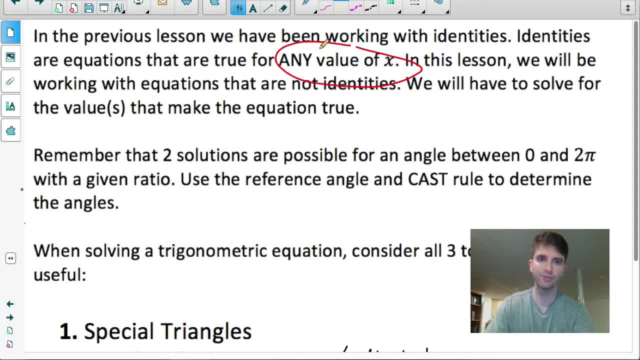 Remember, identities are equations that are true for all values of the variable. What we're going to do for the second half of the unit is look at trig equations that are true for all values of the variable, And then we're going to solve for values that are not identities, meaning they're only true for certain values of the variable. 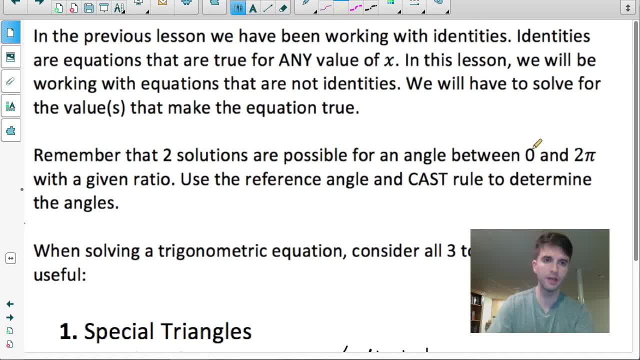 And we're going to have to solve for what values of the variable make that equation true, And we're always going to find the angles that are between 0 and 2 pi. If we didn't restrict the domain, there would be an infinite number of angles that would have any given trig ratio. 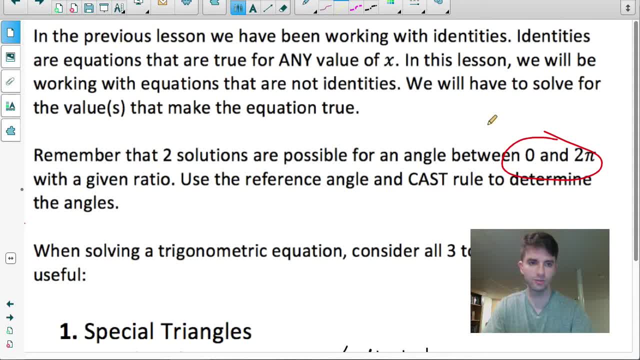 because trig functions are periodic. They have patterns of y values that just repeat over and over and over again. So when solving these equations it's important to remember that between 0 and 2 pi there are often two angles that have any given trig value. 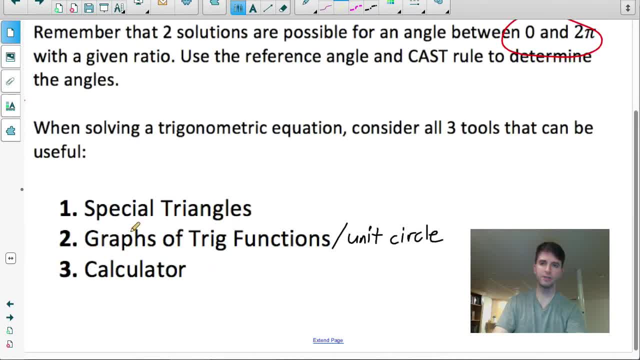 So we're going to have to use our cast rule in combination with these three tools- special triangles, unit circle and calculator- to figure out what angles have each given trig ratio. Now the special triangles and unit circle are going to give us exact answers for the angles. 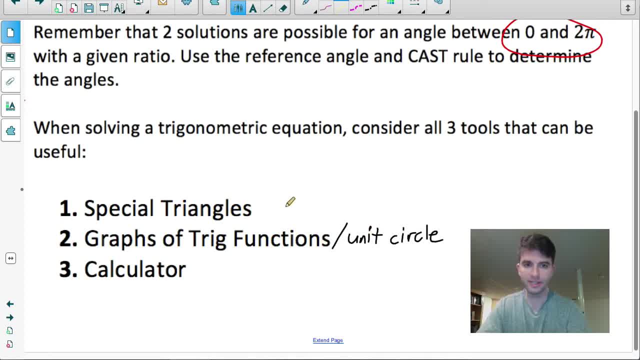 so we'll give preference to those two tools. But if we can't get an exact answer for the angle, then we use our calculator to get an approximate answer using the inverse trig functions. So let me remind you about special triangles. Let's look at the special triangles and unit circle quickly before we do our examples. 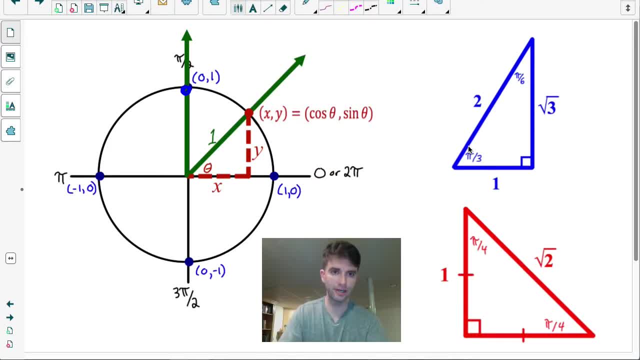 So here are the two special triangles. We have our half-equilateral triangle, angles pi over 3,, pi over 6, and our isosceles special triangle angles pi over 4,, pi over 4.. So here's the unit circle. 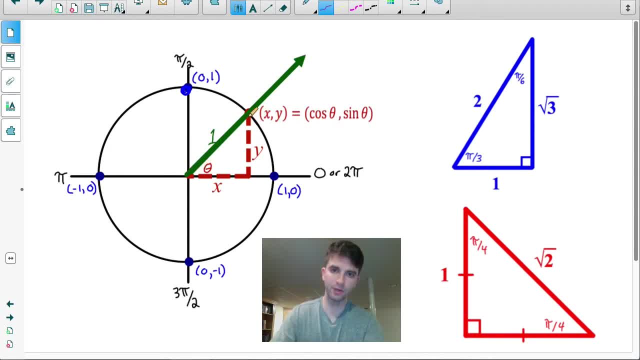 And remember, if we know the x and y coordinate of where a terminal arm intersects the unit circle, then we know the cosine and sine ratio for that angle of rotation. The x coordinate tells us the cosine ratio and the y coordinate tells us the sine ratio. 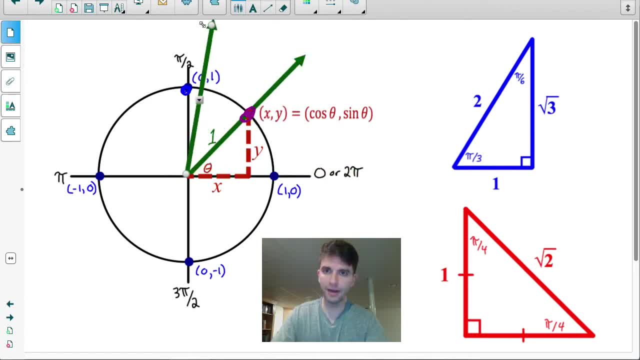 So, for example, if I were to rotate pi over 2 radians- and in this course we're always working in radians- I should mention that If we rotated pi over 2 radians, I know I would be intersecting the unit circle at this point, right here. 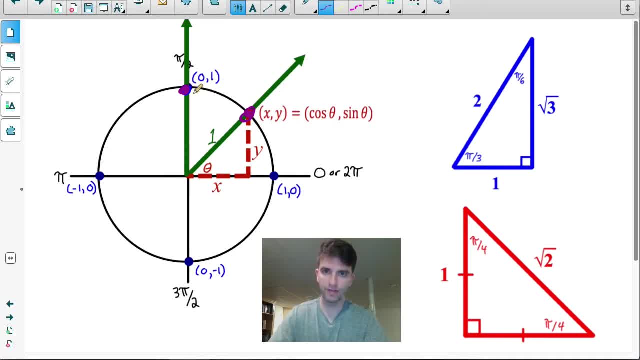 And because it's a unit circle, meaning radius of 1, I know the coordinates of that point are 0 and 1.. The x coordinate would tell me the cosine ratio for the angle of rotation, so cos of pi over 2 must be 0, and the y coordinate tells me the sine ratio. for the angle of rotation. So cos of pi over 2 must be 0, and the y coordinate tells me the sine ratio for the angle of rotation, So cos of pi over 2 must be 0, and the y coordinate tells me the sine ratio for the angle of rotation. 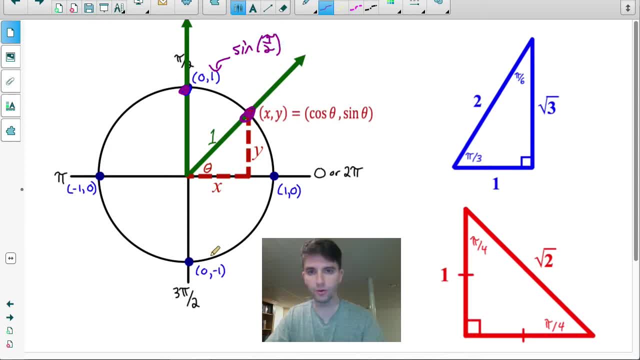 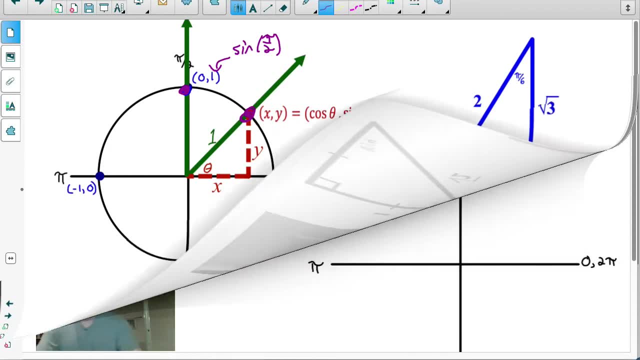 So sine of pi over 2 must be equal to 1.. So, knowing these tools, let's try and solve the four examples we're going to do in this lesson. Let's get going. Example 1 says: find all solutions for cos. theta equals negative root 3 over 2. 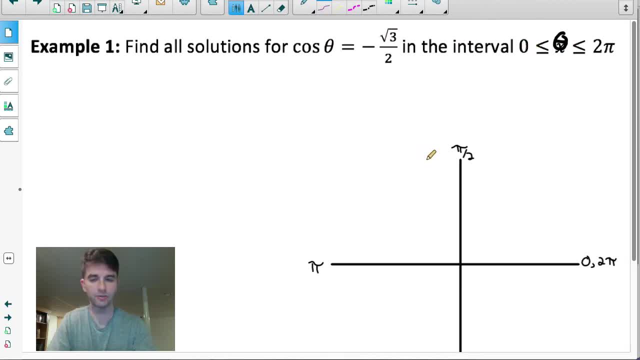 in the interval where theta is between 0 and 2 pi, including 0 and 2 pi. So let me just make sure you understand graphically what we're trying to figure out. So let me show you what cos theta looks like in Desmos and we'll see. 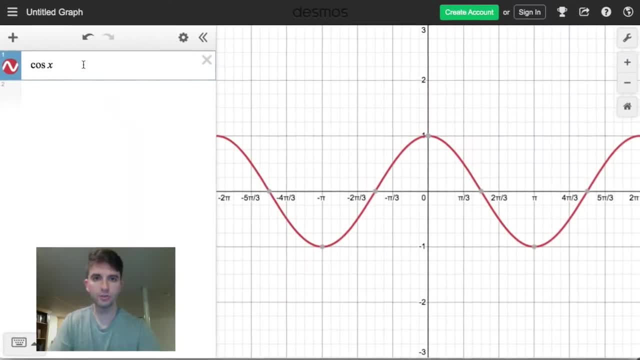 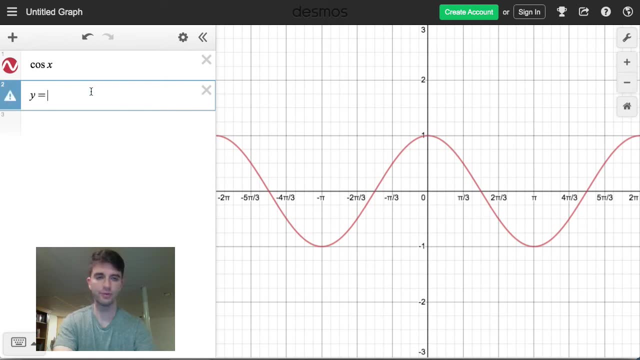 when is it equal to negative root 3 over 2.. So here's a cosine function and we're interested in. when is this cosine function equal to negative root 3 over 2.. So let me just draw a horizontal line through negative root 3 over 2,. 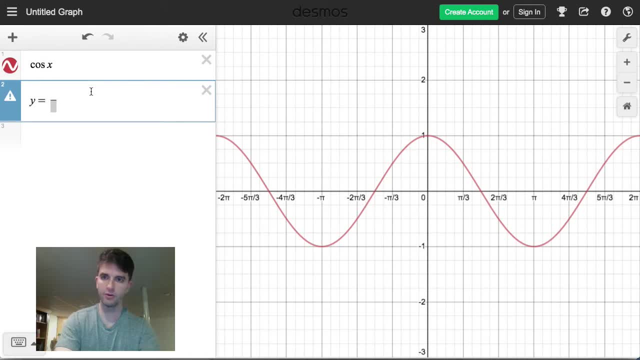 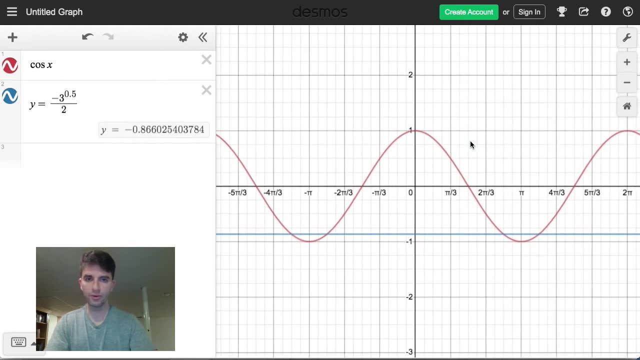 so it'll be easier for us to visualize this. So negative root 3 over 2.. And we want to know when is the cosine function equal to negative root 3 over 2,? so when does the cosine function intersect that horizontal line? It does it right here. 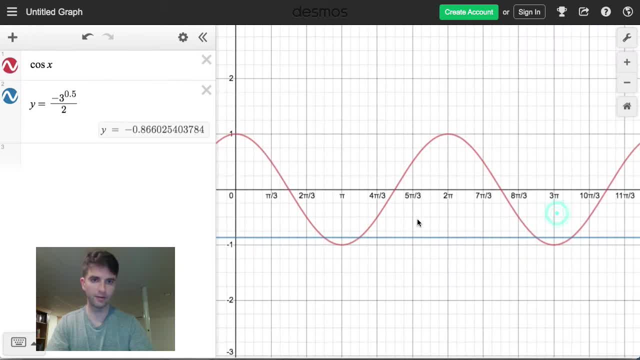 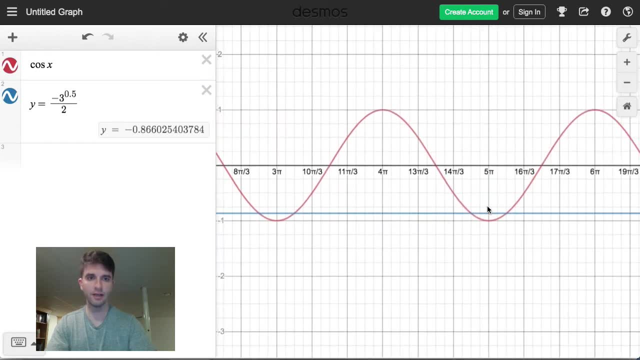 at 5 pi over 6.. Right here at 7 pi over 6.. And then again here at 17 pi over 6.. Here, 19 pi over 6. And notice, there's an infinite number of solutions. 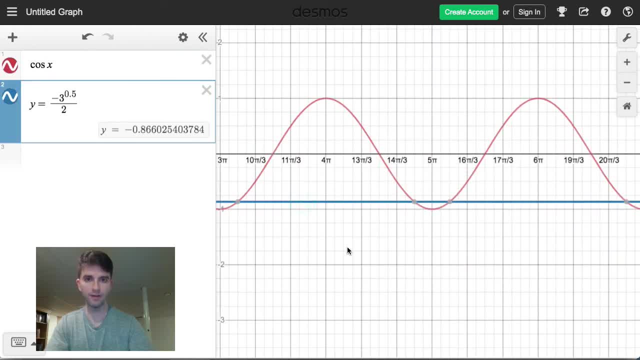 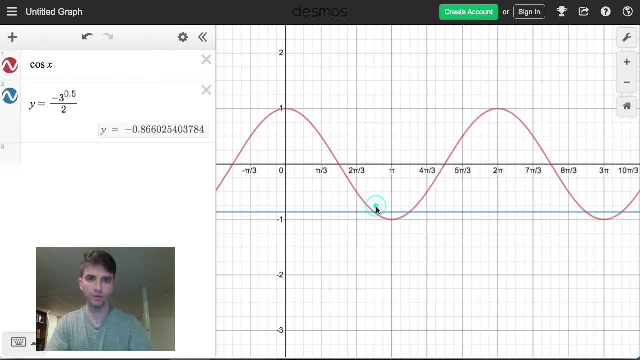 because this function is periodic, right, It's going to have that pattern of y values. it just repeats over and over again. So the question says: well, we only want the answers between 0 and 2 pi, so we only want these two answers. 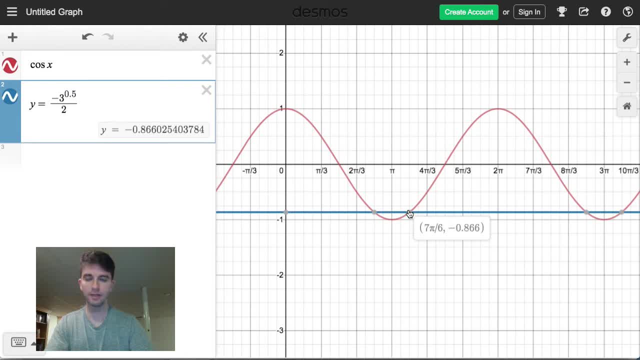 So we have to figure out, well, how are we going to get those answers algebraically? And notice, we were able to get those answers algebraically, but we're not able to get exact answers. for this right, The angle is exactly 5 pi over 6, and exactly 7 pi over 6.. 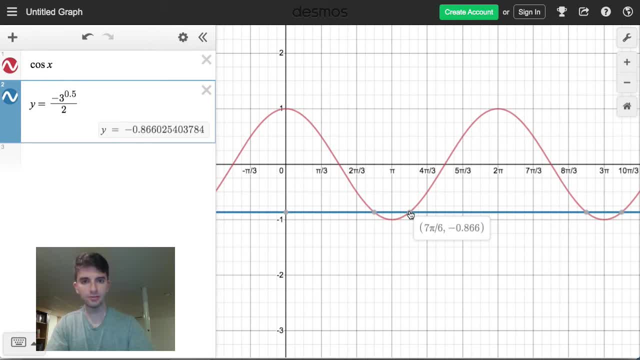 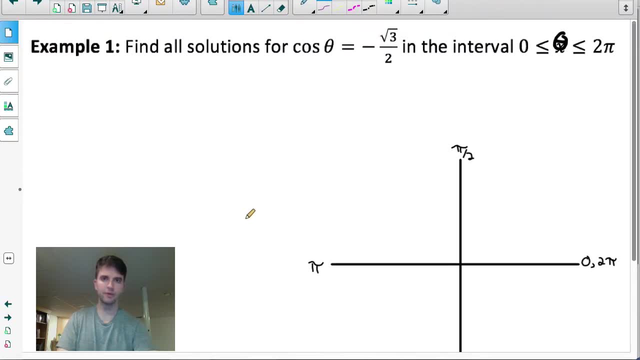 So we're going to be able to get those exact answers by using our special triangles. And how are we going to know how to get both of those answers? Well, notice, if we look at this Cartesian grid I've drawn here. remember, there can be up to two angles between 0 and 2 pi that have any given ratio. 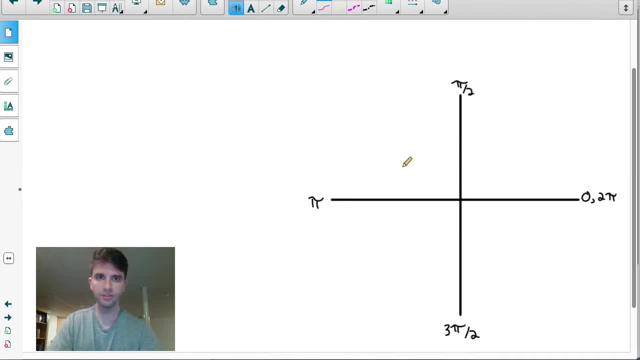 and the cast rule tells us in what quadrant what ratios are positive. So let me just label the cast rule C-A In the question: the cosine ratio has to be negative. Well, where are cosine ratios negative In this quadrant and this quadrant? 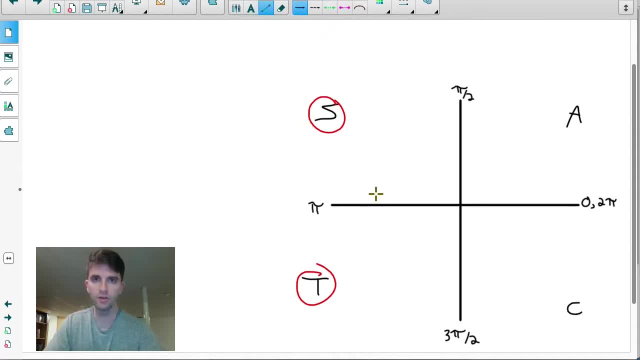 So I know there's going to be an answer in both of those quadrants. So I know there's going to be some angle in both of those quadrants that have that cosine ratio and both of those angles are going to have the same reference angle. 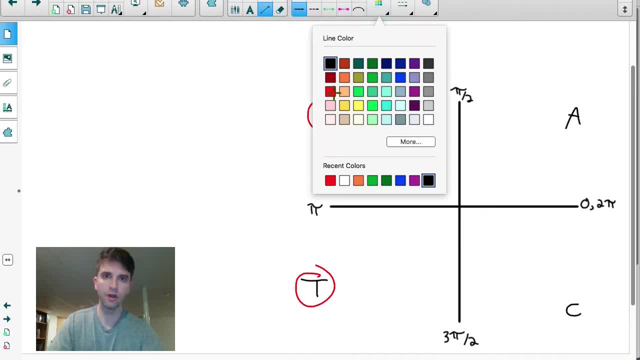 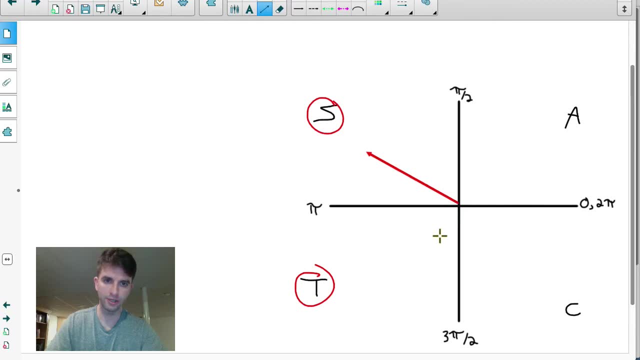 So I could start by drawing a terminal arm in both of those quadrants where the terminal arms have equivalent references. So I could draw a terminal arm here and here. Now I don't know if the measures of those angles are perfect, but I know there is going to be a terminal arm in both of those quadrants. 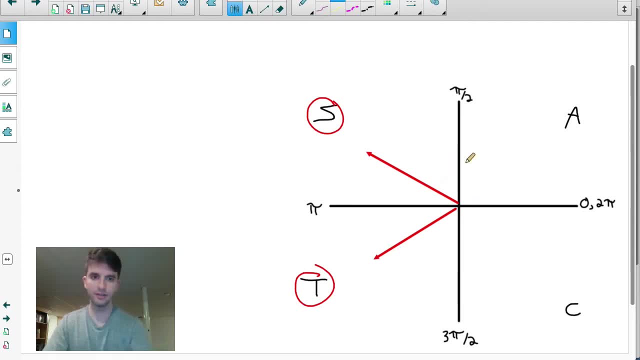 where the angle from positive x-axis to there and the angle from positive x-axis to there are both going to have a cosine ratio of negative root 3 over 2.. And I know these two angles are going to have the same reference angle. I'll label those reference angles beta. 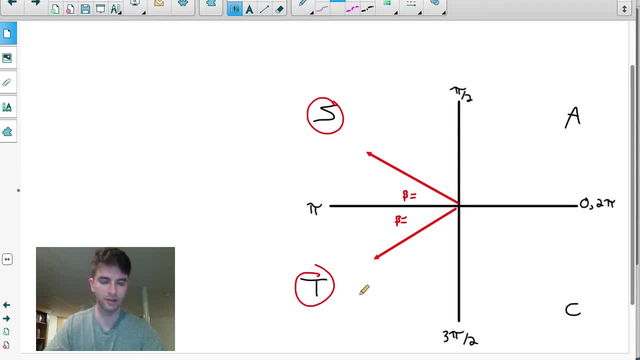 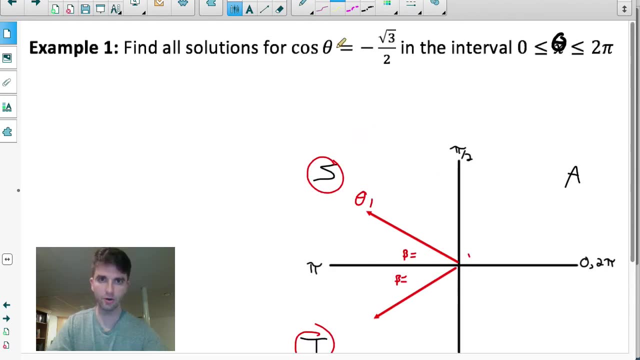 Remember, reference angle is the angle between terminal arm and x-axis And I will call this principal angle. I'll call that theta 1.. We're actually trying to solve for theta the principal angle that has a cosine ratio of negative root 3 over 2.. 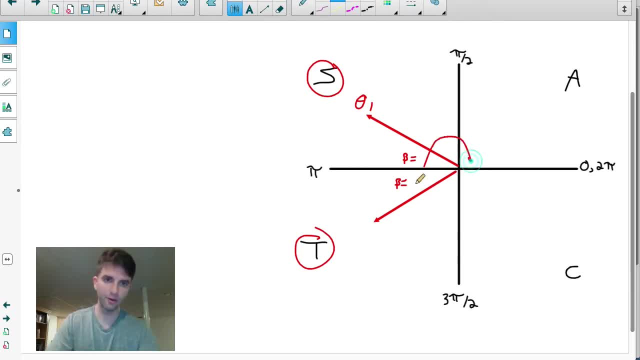 So I need to know what do I have to rotate to get to there, and I also have to know what do I rotate to get to there. So I'll call this one theta 2.. I'm going to get two answers, one in each of the quadrants where cosine is negative. 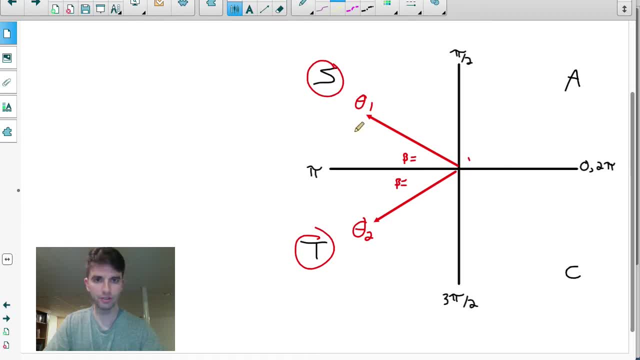 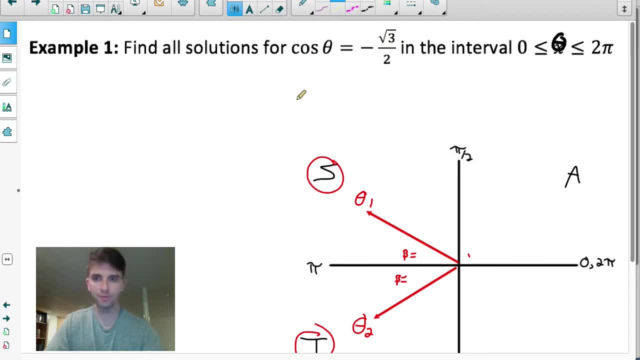 But now I have to figure out. well, what reference angle should I put in both of those quadrants to help me calculate theta 1 and theta 2?? And that's very special. Triangles come in handy. So instead of just blindly asking your calculator what's inverse cos of negative root 3 over 2? 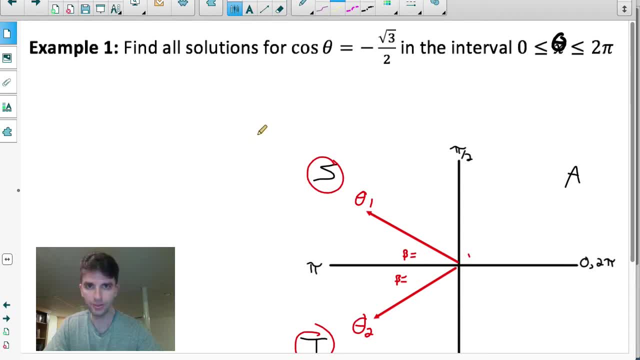 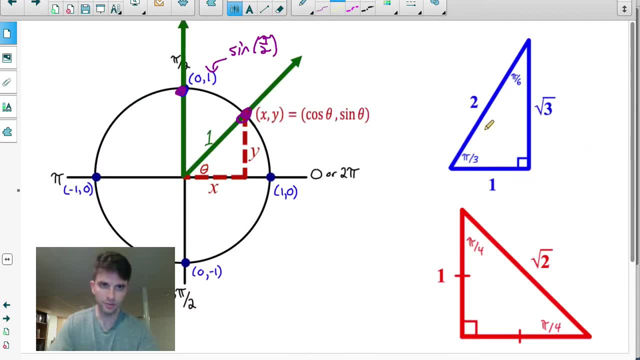 and getting the approximate answer from your calculator. instead, we're going to look to our special triangles and see if we can get an exact answer. Well, in the special triangle notice we could get a cosine ratio of root 3 over 2 if we did cosine of pi over 6.. 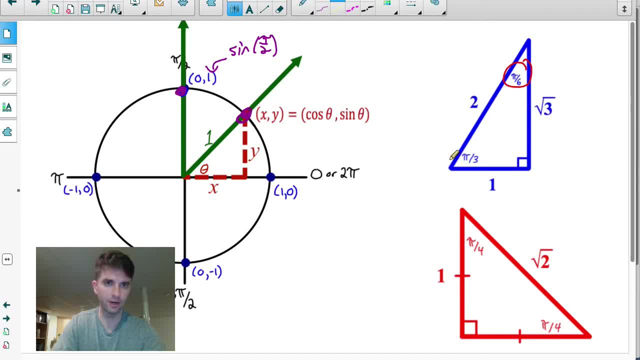 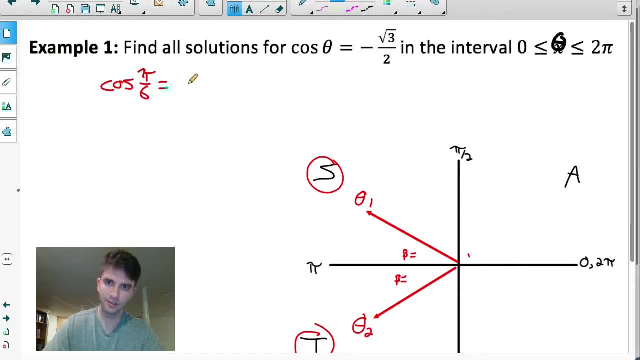 Cosine of pi over 6 equals adjacent root 3 over hypotenuse 2.. I want to make a note of that here. Cosine of pi over 6 equals root 3 over 2.. So what do I do with that information? 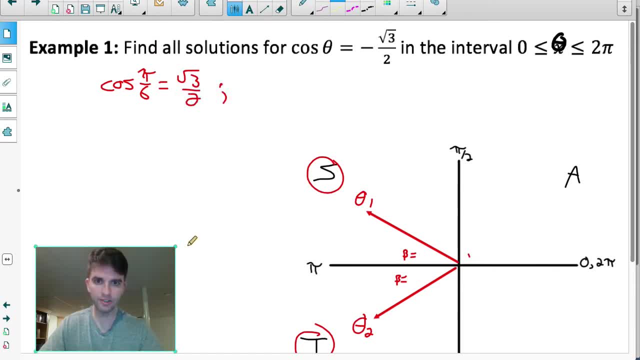 Well, if I were to place a reference angle of pi over 6 in quadrant 2 and 3, I would actually get a cosine ratio of negative root 3 over 2.. So place reference angle of pi over 6, of pi over 6,. 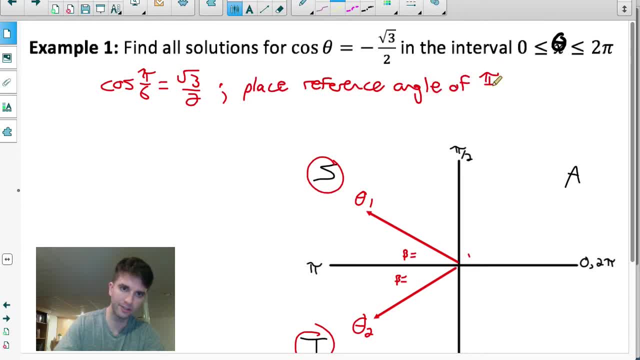 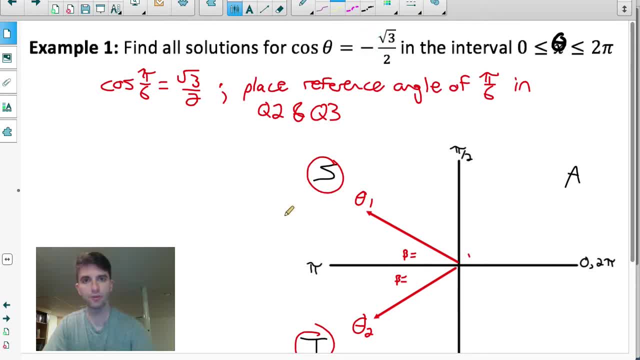 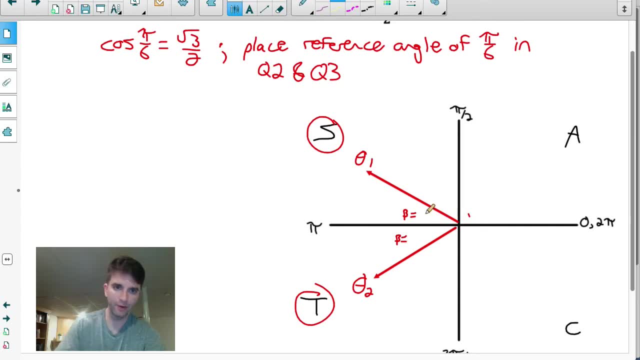 3, because those are the two quadrants where cosine is negative. so place the reference angle on those two quadrants and once we do that we can solve for theta 1 and theta 2, so I now know my reference angle is pi over 6, so I can put that reference angle. 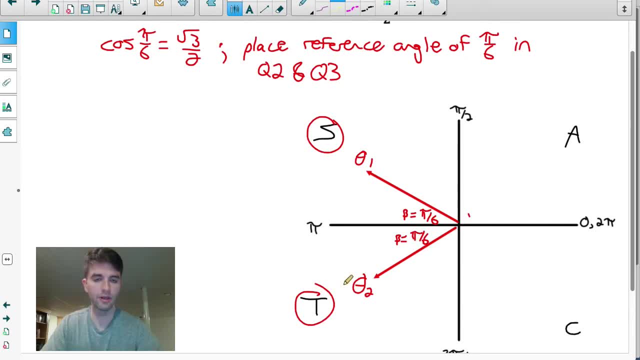 beta as pi over 6 in both of those quadrants. and now I can calculate theta 1 and theta 2, so theta 1, I have to figure out how far do I have to rotate from the initial arm to here. well notice, I didn't go a full pi, I went pi over 6 short of that. so do pi minus. 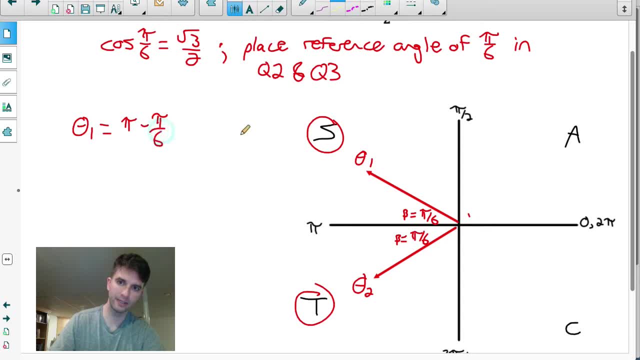 pi over 6, and we get the principal angle: theta 1. So 6 pi over 6 minus 1 pi over 6 is 5 pi over 6, and theta 2,. notice, we went past pi by pi over 6, so I do pi plus pi over 6,, so pi plus pi over 6,, so that's 6 pi over 6 plus. 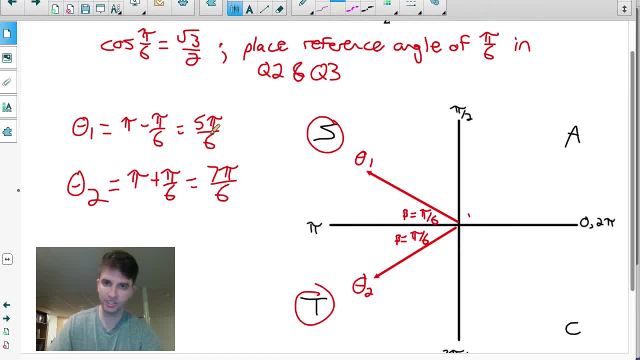 1 pi over 6,, that's 7 pi over 6.. So notice, those are the two angles that Desmos showed us had the cosine ratio of negative root, 3 over 2, and we were able to calculate them using our special triangles and castrules. 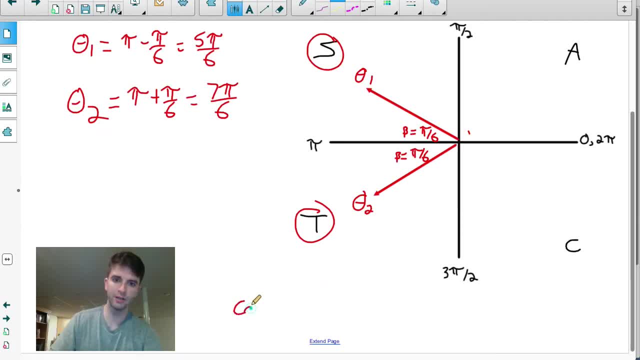 So let me just summarize what we figured out. We figured out that cosine of 5 pi over 6 is equal to cosine of 7 pi over 6, and those are both equal to negative root 3 over 2.. And we could check this on our calculator to make sure it's right. 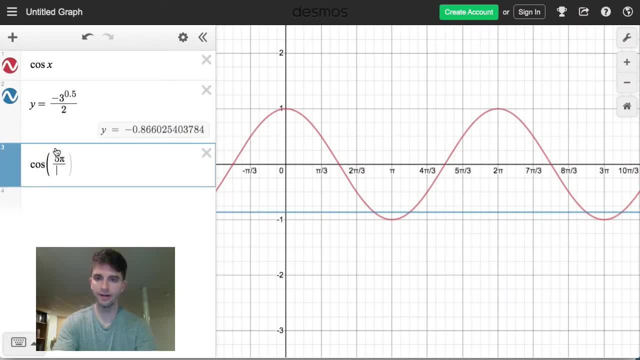 Let me just show you So we could evaluate cosine of 5 pi over 6,- make sure you're in radian mode- and also evaluate cosine of 7 pi over 6. And both of those should have the same approximate value that negative root 3 over 2 had right. 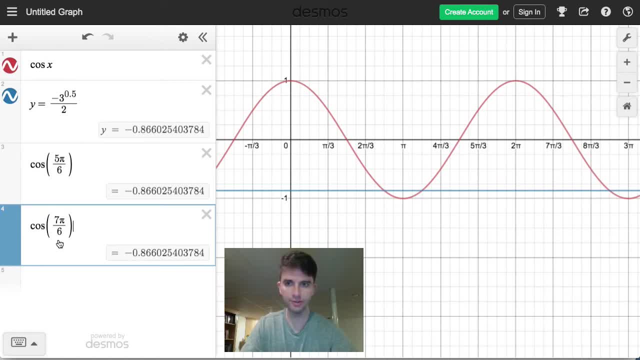 So we just showed that these three things are equivalent, and that's what we tried to do. We figured out the angles- 5 pi over 6 and 7 pi over 6, that have a cosine ratio of negative root 3 over 2.. 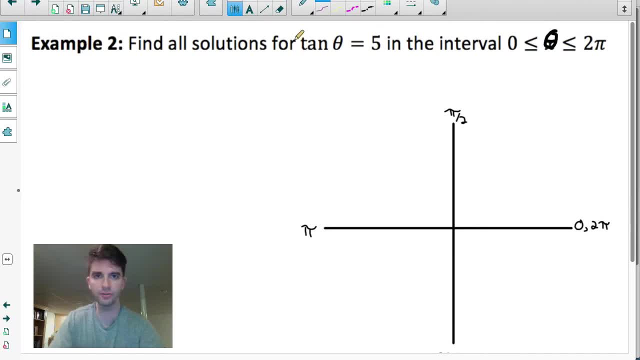 Let's move on to example 2.. Example 2 says: find all solutions for tan. theta equals 5 in the interval where theta is once again between 0 and 2 pi. So this equation is going to be a little bit different than example 1, because we're not. 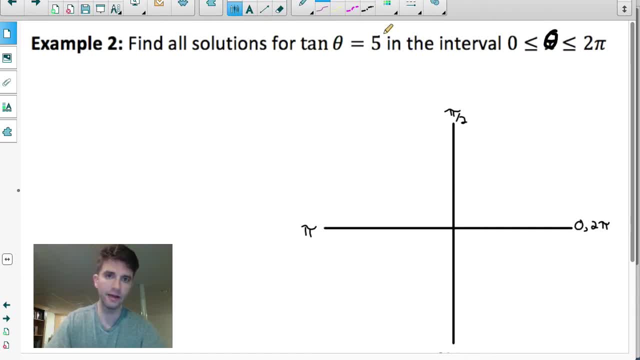 going to be able to get exact values. Okay, We're going to be able to get exact values for the angle that creates a tan ratio of 5.. And why can't we get an exact value? Well, a ratio of 5, right, and for tan it would be an opposite over adjacent ratio. 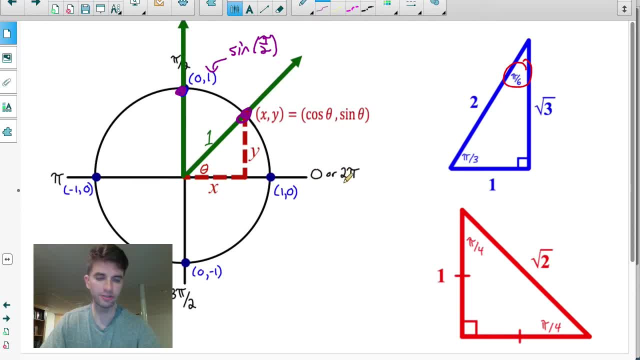 can't be created from a special triangle. Let's look back at the special triangles. There's no way I can create an opposite over adjacent ratio of 5 from any of my special angles, So I'm not going to be able to get an exact answer for theta in the equation tan theta. 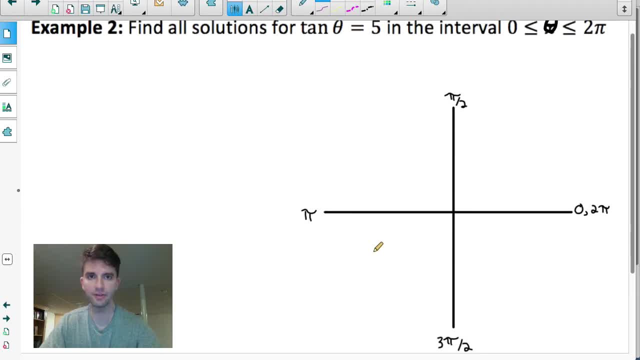 equals 5.. So we're going to have to rely on our calculator to give us the approximate answers. Let's start by the same way we did last question right? Let's label our cast rule and figure out what two quadrants are we going to get answers. 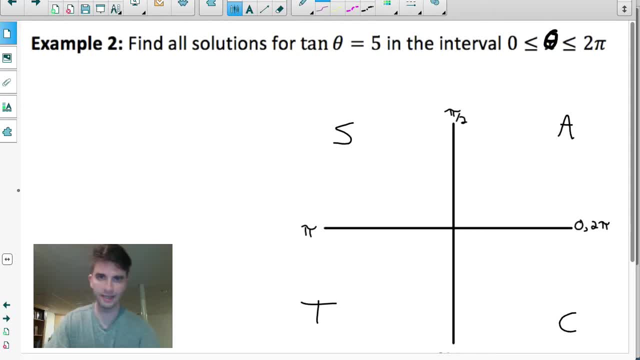 in. Well, we have a tan ratio that is positive where a tan ratio is positive in this quadrant and this quadrant. So I know there are going to be angles of rotation in both of those quadrants that have a tan ratio of 5.. 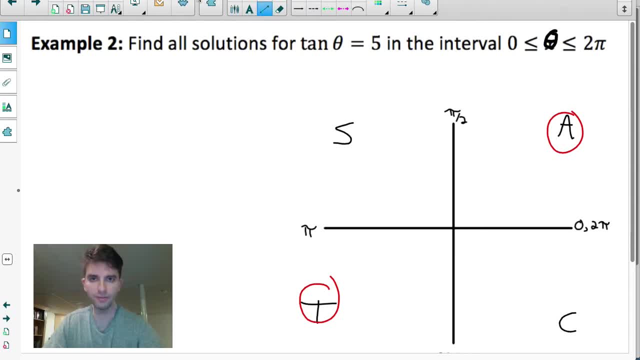 And I know those angles are going to have the exact same reference angle, So I can draw terminal arms in both of those quadrants that have equivalence. Okay, Terminal arms that have equivalent reference angles. I don't know what the reference angle is yet, but I can draw the terminal arms anyways. 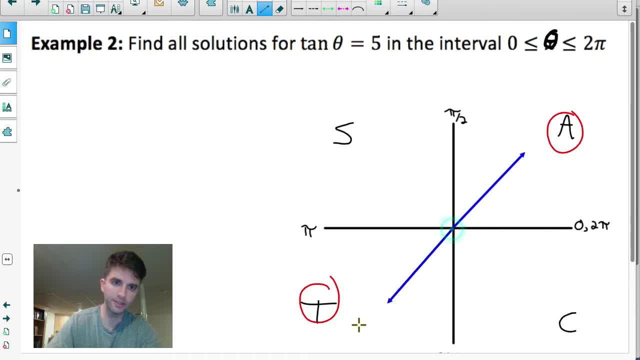 So I'll draw a terminal arm in quadrant 1 and 3.. And both of those terminal arms, in order for them to have the exact same tan ratio, must have the same reference angle. So I'll just label those reference angles beta. 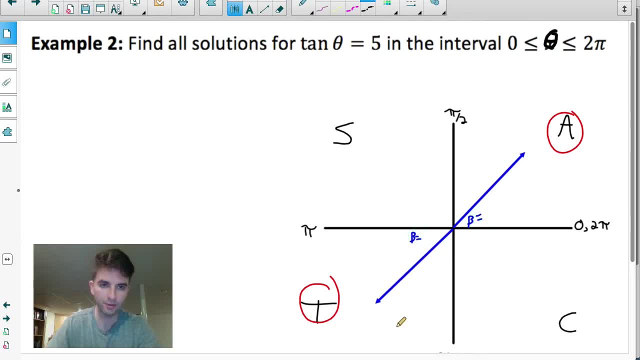 I don't know what the measures of those reference angles are yet, but I'll label them beta for now, And we'll have to solve for those reference angles. And let me label the principal angles. I'll label them theta 1.. Okay, 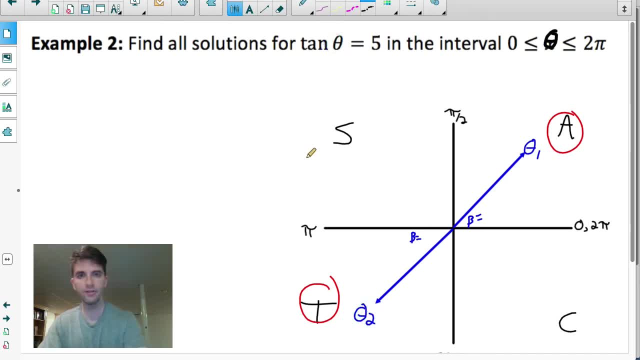 And theta 2.. Right, I'm going to get two answers for theta that give a tan ratio of 5.. Now, since I can't use my special triangles to figure out the reference angle, what I'm going to do is I'm going to get my calculator to give me either theta 1 or theta 2.. 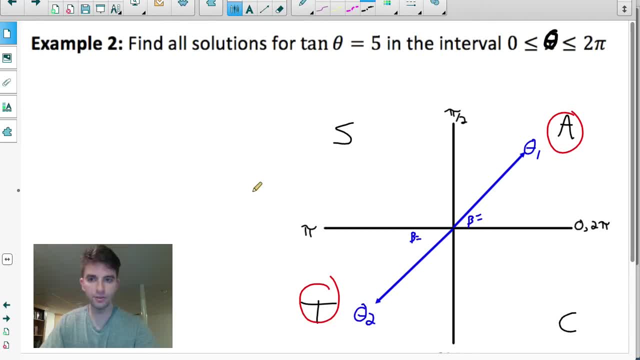 Now the calculator. it will always give you the smaller of the two. However, it can express the angle with the smallest possible value, or I should say a value as close to 0 as possible. that's the one the calculator will give you. 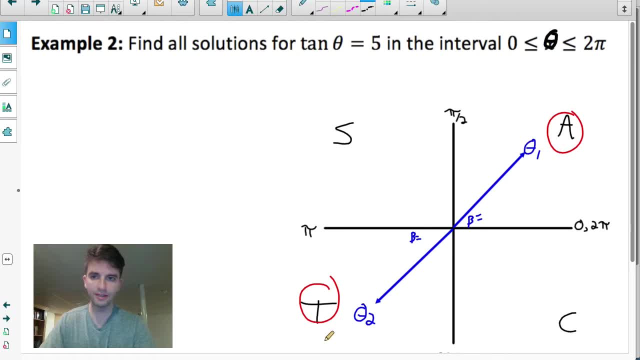 So the calculator will? It will either give you theta 1 or theta 2.. It will give you one of the principal angles And in this case it will give us theta 1, because that's the smaller of the two angles. So how do we ask our calculator for an angle that has a given ratio? 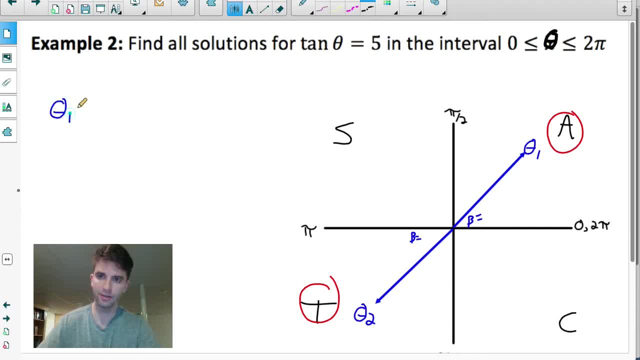 Well, we use the inverse trig ratios. So I can calculate theta 1 by doing inverse tan of the ratio. So inverse tan of 5 will tell me the angle from positive x-axis to here. So let's type this in on our calculator. 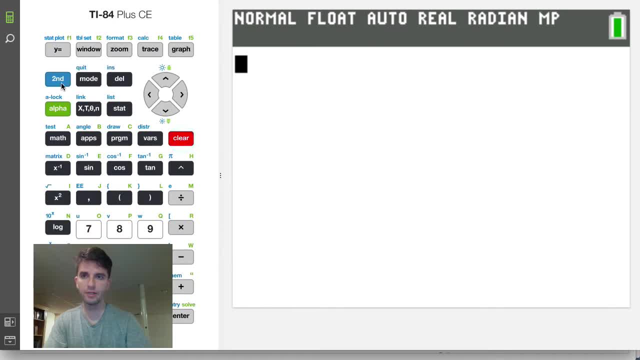 You should always make sure that you're in radians. I'm in radian mode for this course, so I'm in radian mode And now I can do inverse tan of 5, and my calculator will give me the approximate answer And I'll round it to two decimal places. 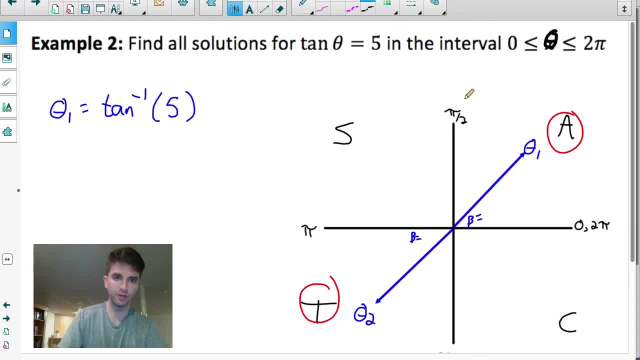 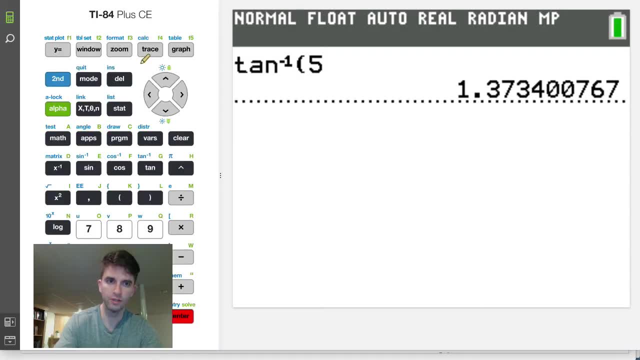 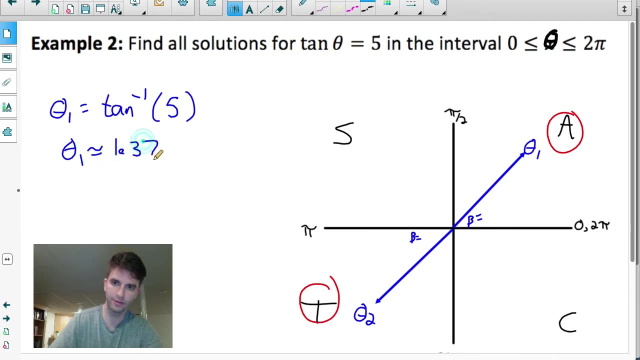 So 1.37 radians. That's between 0 and pi over 2.. So I know I'm in the correct quadrant. So it gave me theta 1 was 1.37 radians. So theta 1 is approximately equal to 1.37 radians. 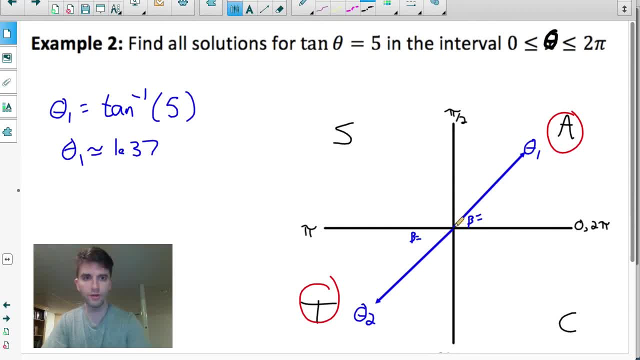 So that's the angle from here to here. And since we're in quadrant 1, the principal angle and the reference angle are the same. The reference angle is also the angle between here and here. So we've also, by finding theta 1, we've also found the reference angle: 1.37.. 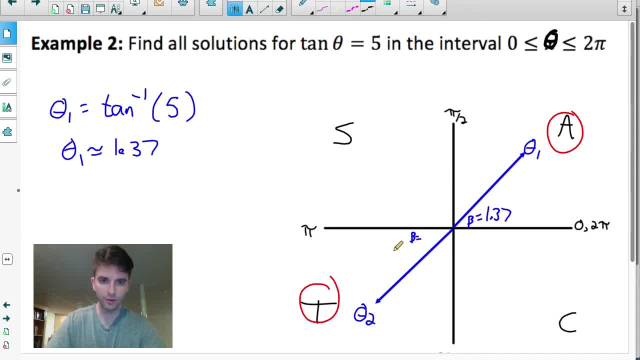 So what I need to do is place that reference angle in the other quadrant where tan is positive. So place it here, And then I can use that reference angle to be able to calculate the principal angle from here all the way around to there. Notice, 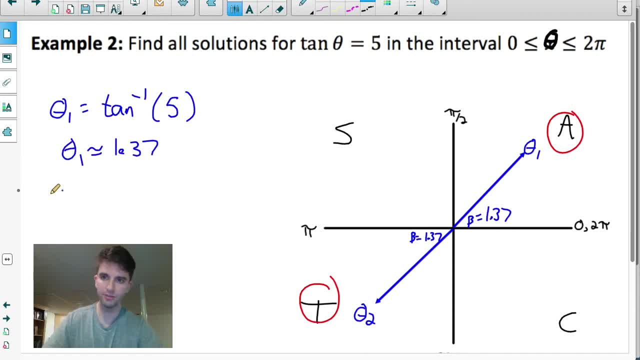 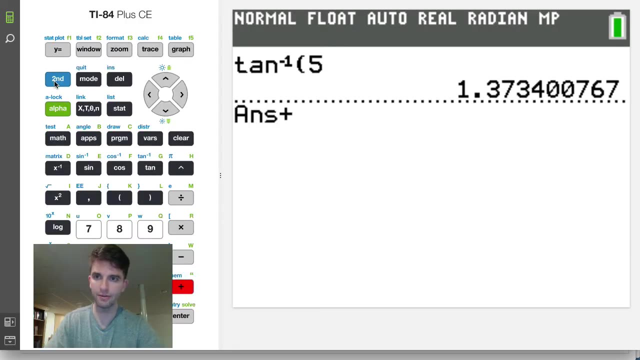 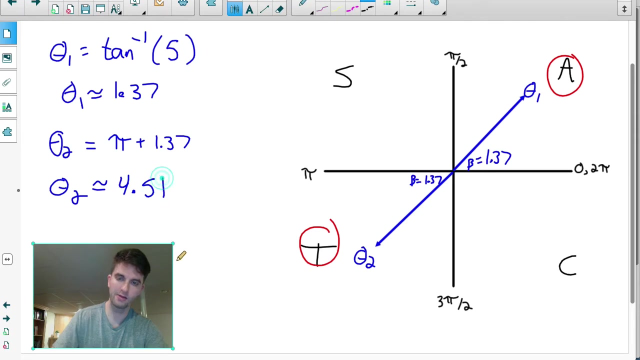 It's past pi by 1.37.. So theta 2 would be equal to pi plus that reference angle, 1.37.. So theta 2 would be approximately equal to: let's add pi to that reference angle and we get 4.51 approximately. 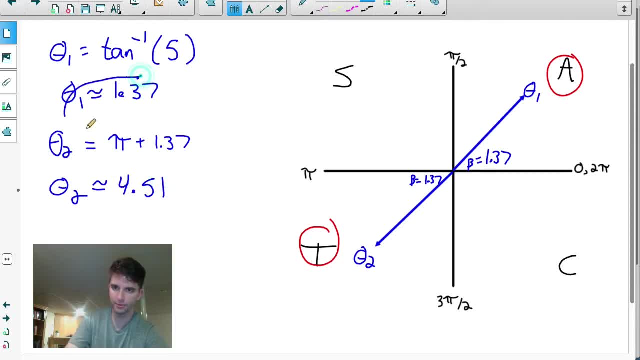 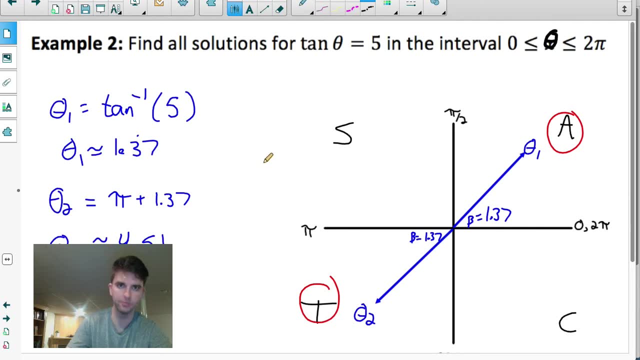 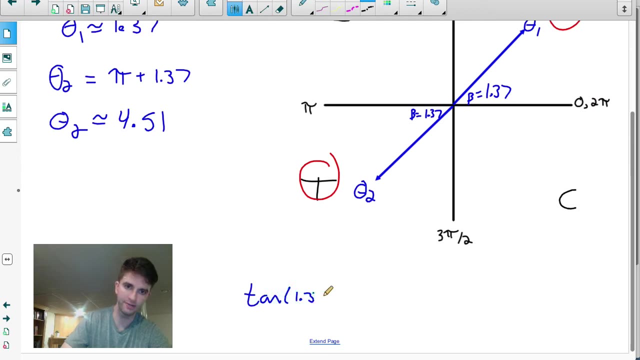 So what we have figured out is that tan of 1.37 radians And tan of 4.51 radians are both approximately equal to 5.. So I could write my concluding statement at the bottom here: Tan of 1.37 equals tan of 4.51, which equals 5.. 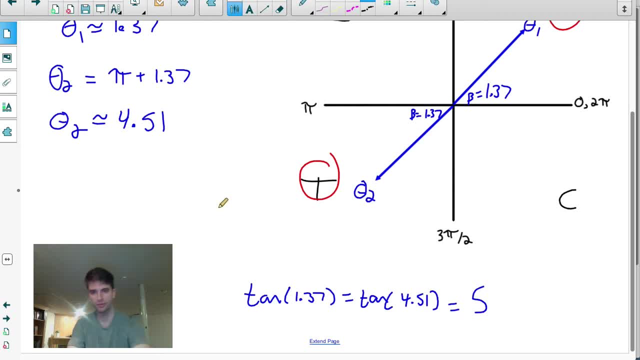 They both have tan ratios of about 5.. Now, if we check these answers, they're not going to be exactly equal to 5, because we've done some rounding, But they should be pretty close. They should be around, you know, 4.51.. 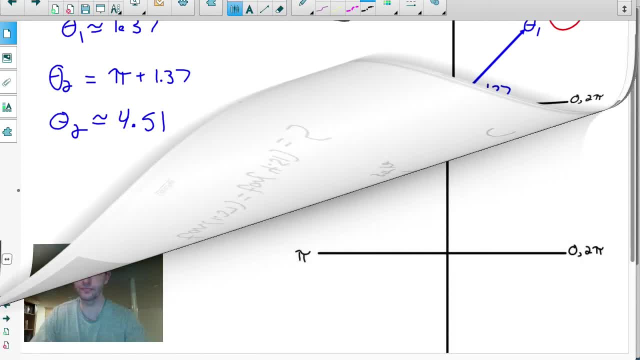 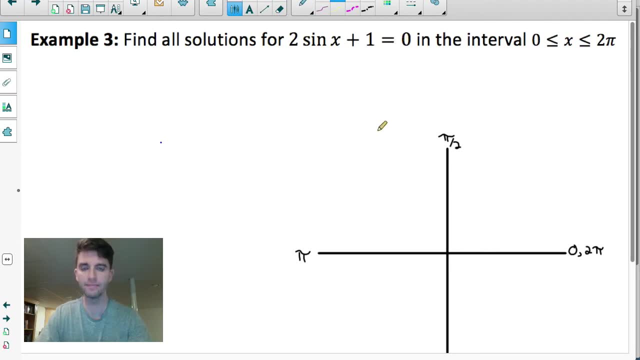 4.9.. All right, let's move on to example 3.. Example 3, find all solutions for 2 sine x plus 1 equals 0 in the interval where x is between 0 and 2 pi. This example is slightly different than the first two because the trig function is not. 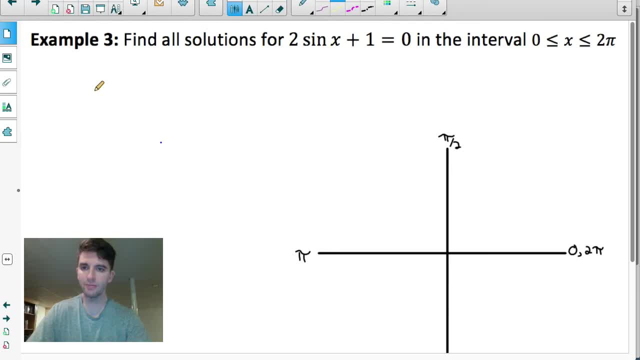 isolated. Sine x is not by itself, So we have to start by isolating it. So I would subtract the 1 to the other side, So I would have 2: sine x equals negative 1. And then divide the 2.. 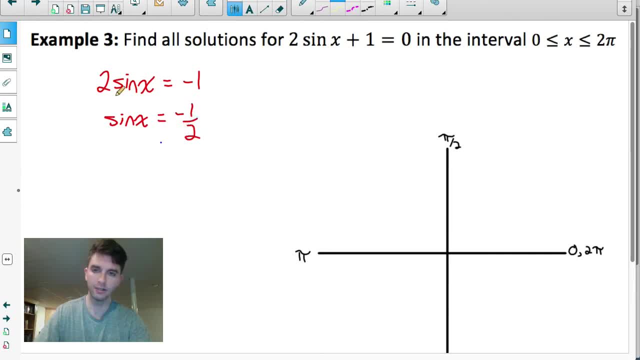 So sine x equals negative 1 over 2.. Now the trig function is isolated and I can figure out what angle has a sine ratio of negative 1.5.. Well, maybe we should start by labeling our cast rule and figure out what two quadrants 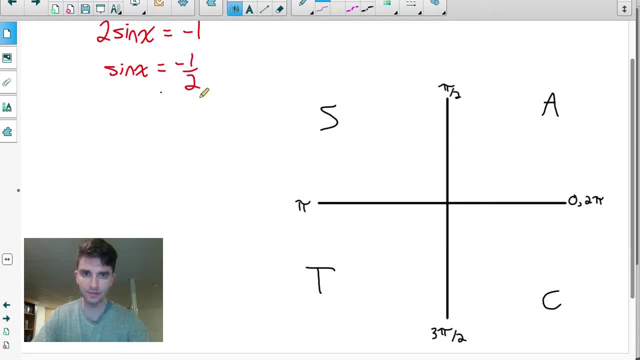 we're going to find our answers in. Since we have a negative sine ratio, my answers are going to be in the two quadrants where sine is negative, So quadrant 3 and quadrant 4.. And I know, in those quadrants, whatever the angles are that have this trig ratio of negative. 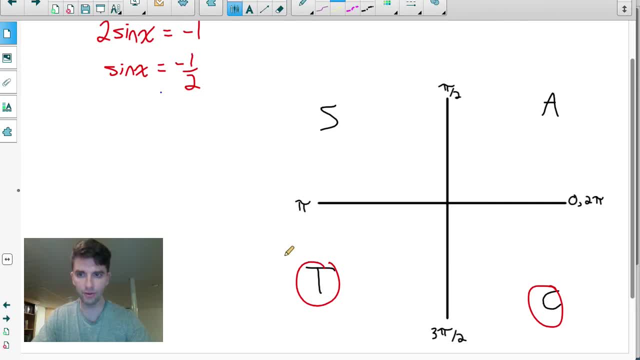 1.5.. Those angles are going to have the same reference angle. That's the only way they can have the exact same trig ratio. So I could draw principal angles in both of those quadrants that have the same reference angle. So I'll draw one in quadrant 3.. 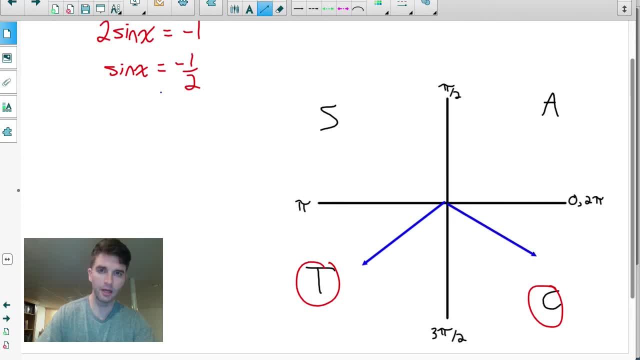 And I'll draw another one in quadrant 4.. And whatever I have to rotate to get to that terminal arm and to get to this terminal arm are going to be the angles that satisfy this equation. So I'll call this one angle 1 and this one angle 2.. 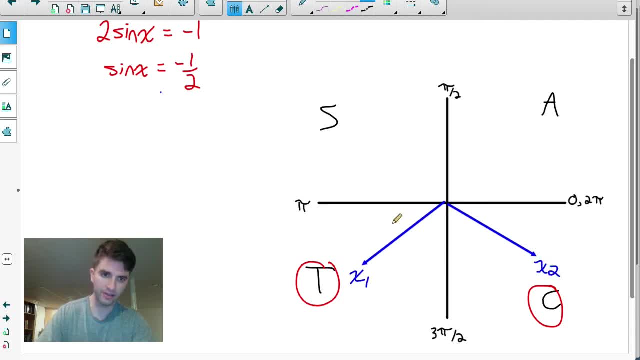 Now both of these angles, like I said, are going to have the same reference angle And, like I said before, don't just automatically start by asking your calculator for an angle by doing inverse sine of negative 1.5.. The calculator will give you, it'll actually give you this principal angle as a negative. 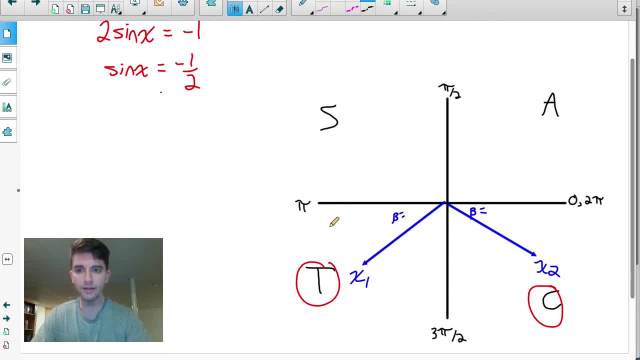 angle, but it would give it to you as an approximate value. We don't want that if we can get an exact value using a special triangle. So we're going to call this one angle 1 and this one angle 2.5. 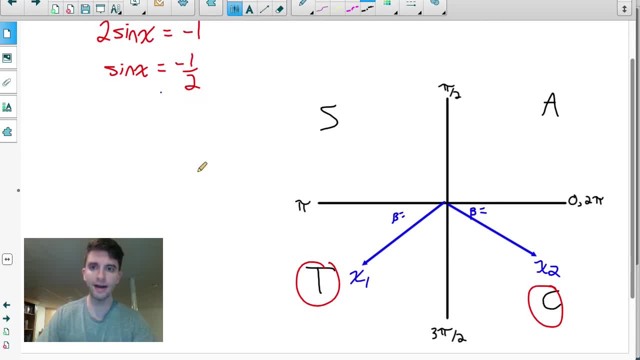 So we have to think: can we make a ratio of a half from a special triangle? So remember your special triangles. Remember this half equal lateral special triangle: the pi over 3, pi over 6,, 2, 1, root 3.. 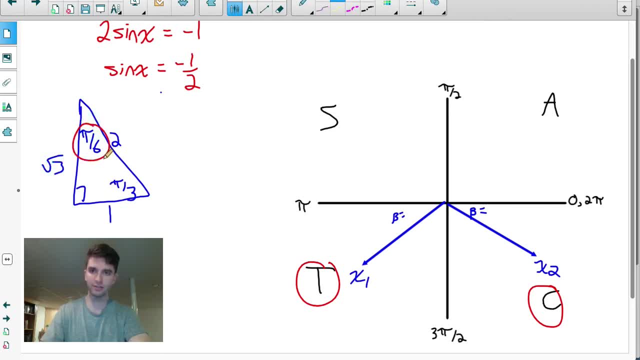 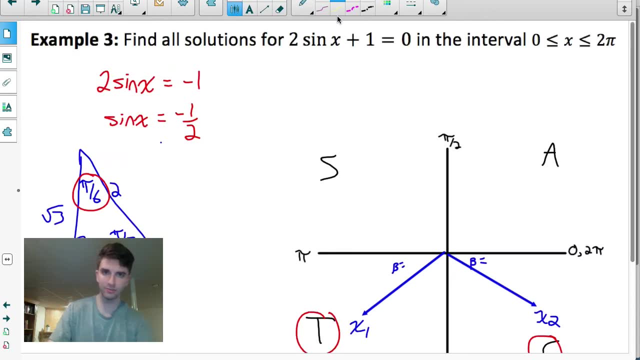 You could make a sine ratio of a half from this reference angle right. Sine of pi over 6 equals opposite over hypotenuse 1 over 2.. So what that tells me? Let me just jot this down. Since sine of pi over 6 equals positive a half, if I place the reference angle pi over 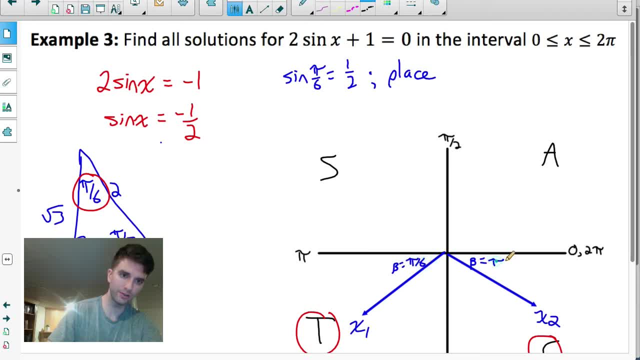 6 in these two quadrants, the quadrants where sine is negative, I will get the ratio of negative a half. So place reference angle pi over 6 in quadrant 3 and 4, right, I'm doing quadrant 3 and 4.. 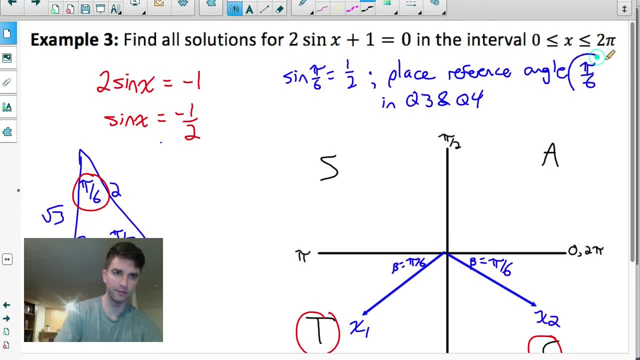 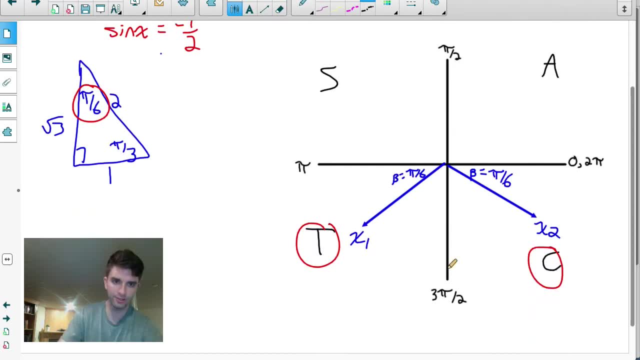 Because I want a negative sine ratio And I'm doing pi over 6, because sine of pi over 6 creates a sine ratio of a half. So placing that reference angle in these two quadrants creates a sine ratio of negative a half. So now I just have to figure out well, what is the principal angle to each of those terminal. 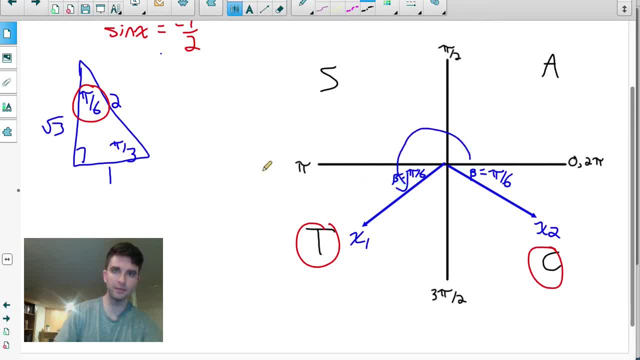 arms. So I need this angle. Notice I went past pi by pi over 6. So I could say: x1 equals pi plus pi over 6. And that gives me so 6 pi over 6 plus 1 pi over 6.. 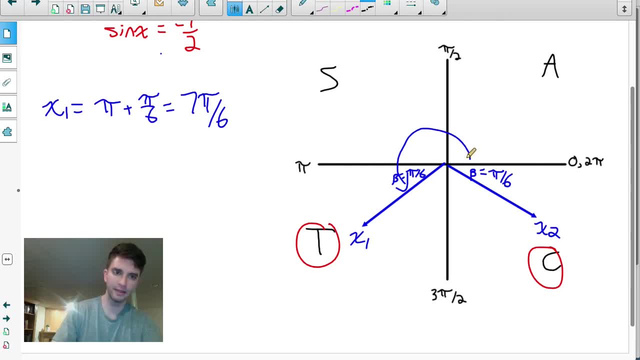 That's 7 pi over 6.. And angle 2, notice I didn't go a full 2 pi. I fell pi over 6 short of going 2 pi. So to get angle 2, all I have to do is do 2 pi minus that pi over 6 reference angle. 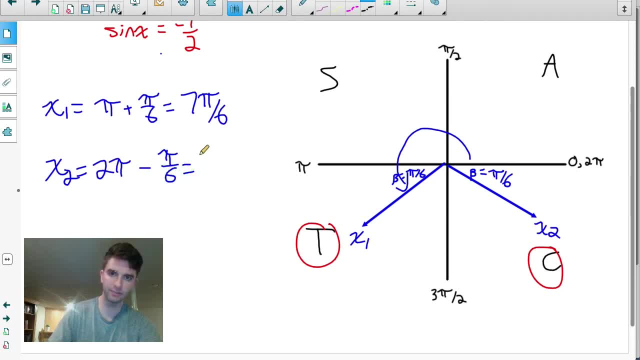 So 2 pi. think of that as 12 pi over 6.. 12 pi over 6 minus 1 pi over 6 is 11 pi over 6.. So these are my two answers: 7 pi over 6 and 11 pi over 6.. 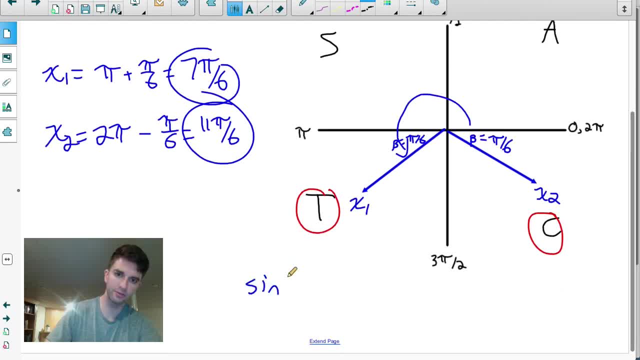 Those are the two angles that have a sine ratio, So sine of 7 pi over 6 and sine of 11 pi over 6. both have that sine ratio of negative a half And once again I would encourage you to actually test these out on your calculator. 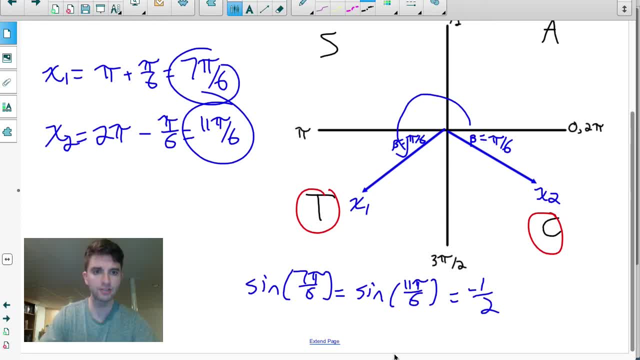 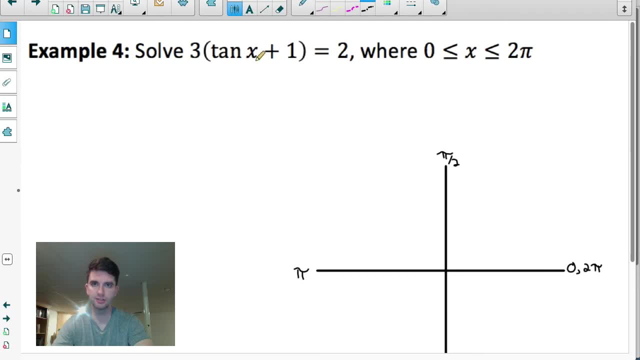 Type sine of 7 pi over 6. Type sine of 11 pi over 6.. Make sure you get negative 1 over 2.. Example 4.. This is the last example. we're going to do So. 3 times 10 of x plus 1 equals 2.. 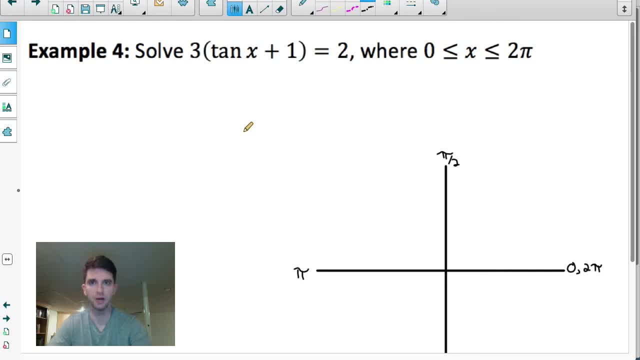 And we want all the answers for the angle that are between 0 and 2 pi. So let's start by isolating this tan function. So when we rearrange this, remember to do bed mass in reverse. We'll do the stuff in the brackets last. 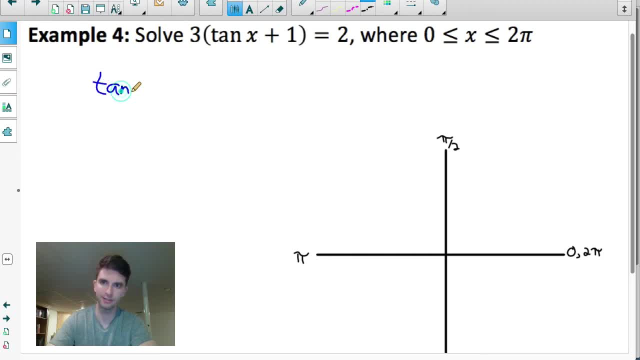 Let's start by dividing the 3 over. So I'll have tan of x plus. So I'll have tan of x plus 1 equals 2 thirds, And now subtract the 1.. So tan of x equals 2 thirds, And now subtract the 1.. 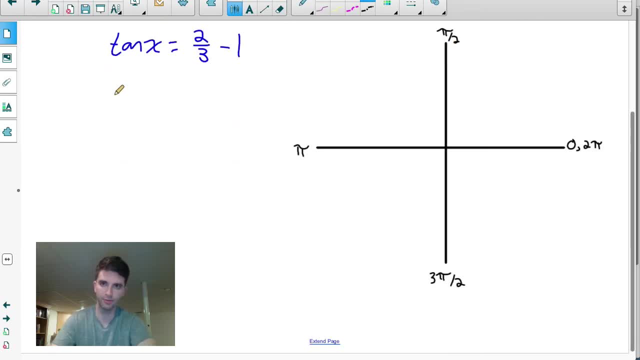 So tan of x equals 2 thirds minus 1.. So 2 thirds minus 3 thirds, That is negative 1 third. Now I need to figure out what angles between 0 and 2 pi have this tan ratio of negative a third. 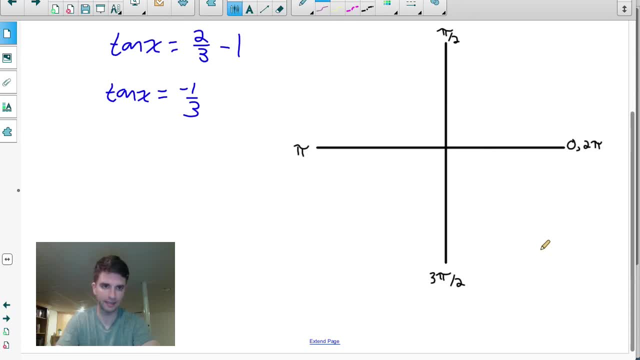 Well, let's start by figuring out in what quadrants am I going to find angles that have a negative tan ratio? So label your cast rule. The cast rule says tan is positive in quadrant number 1 and 3. So therefore, tan would be negative. 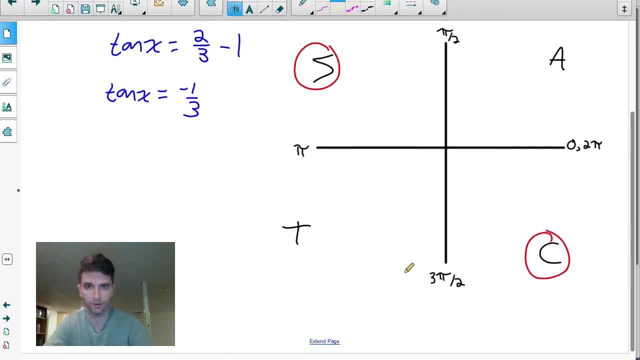 So tan would be negative in quadrants 2 and 4.. So in those quadrants I'm going to find angles that have this tan ratio And those angles would have equivalent reference angles. So let me just draw terminal arms in those two quadrants that have equivalent reference. 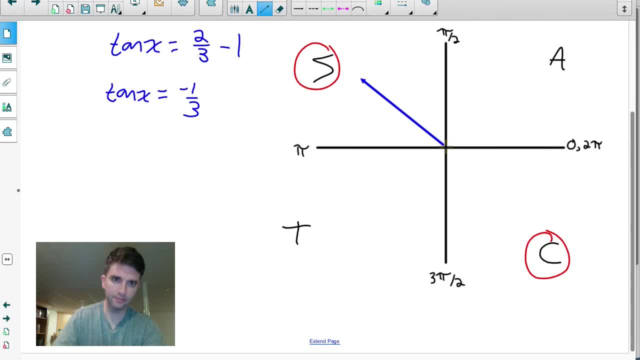 angles And I don't know exactly what the reference angles are, but I'm going to do my best to make sure it looks like those reference angles have the same measure And I'll label those reference angles beta. So I've got beta there and beta here. 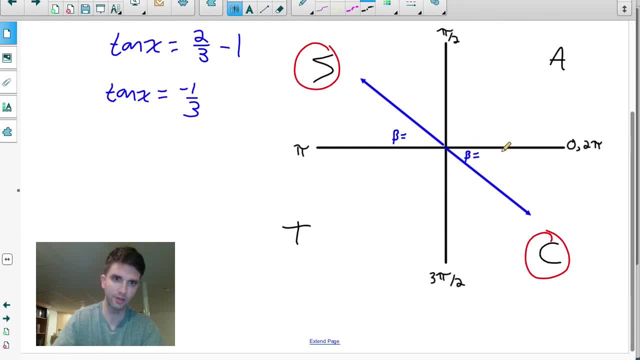 Okay, reference is always between terminal arm and x-axis, So between terminal arm and x-axis they have equivalent, related acute angles called reference angles. I'm going to get two answers. One of the answers is going to be how far I rotate to get to that one. 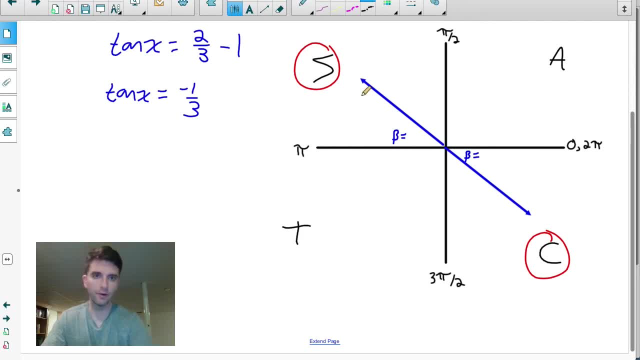 And the other one is: how far do I rotate to get to that one? Now, I'm actually going to label this one my first answer and this one my second answer, And I'm only doing it in that order because I know the calculator is actually going to. 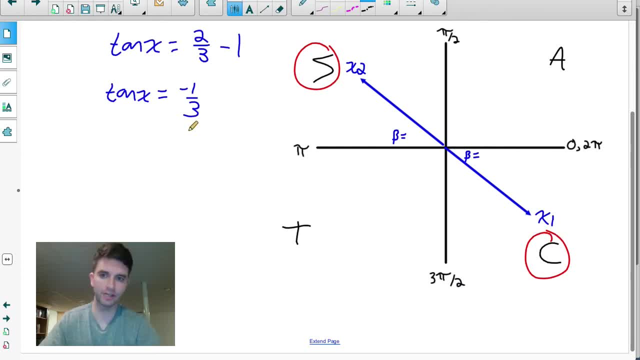 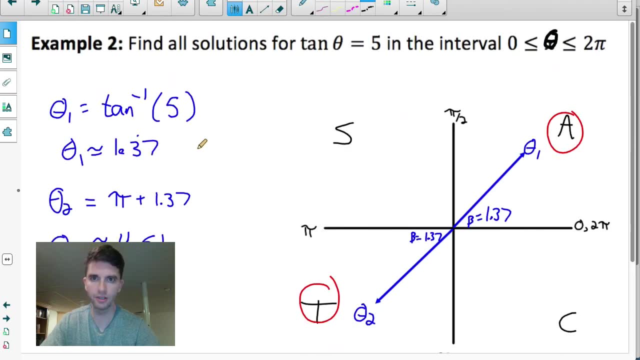 give me this answer. Oh, and I should mention, We're going to have to use our calculator for this. Okay, For this question, to get approximate answers right, We can't make a ratio of a third from a special triangle, From neither of these special triangles. there's no angle that would give me an opposite over. 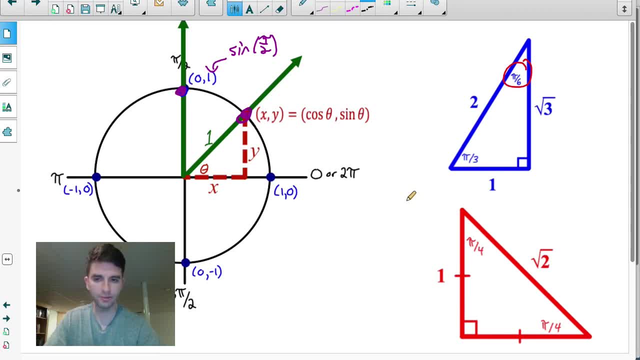 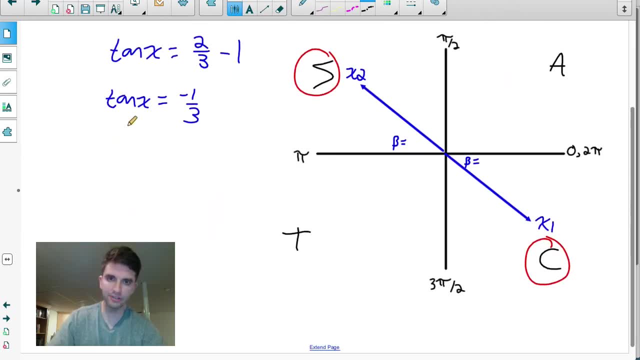 adjacent ratio of one over three. So it's not possible to get an exact answer for an angle for this question. So we'll rely on the calculator to get an approximate answer. To get the first answer we can do, inverse tan of the ratio. 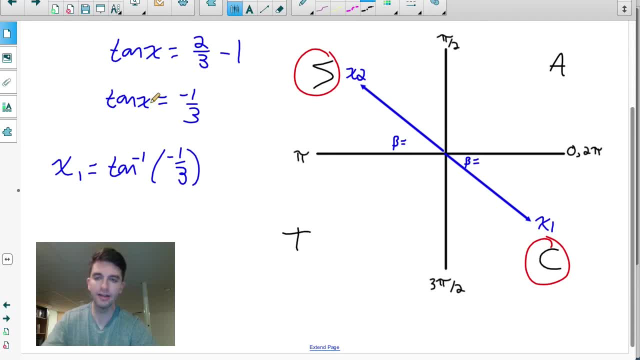 We'll give me one of the principal angles that has that exact tan ratio. Now, however, the calculator will always give you the angle that is as close to zero as possible, So it's going to give you this angle expressed as a negative angle, which means clockwise. 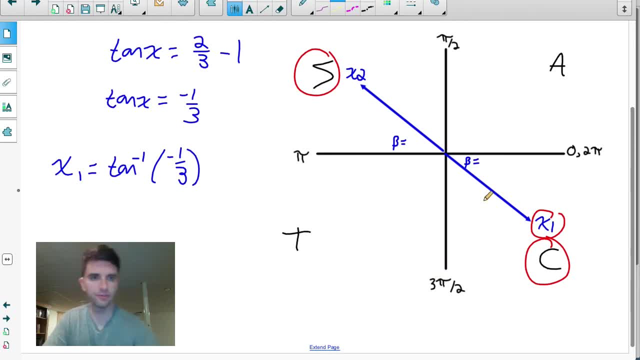 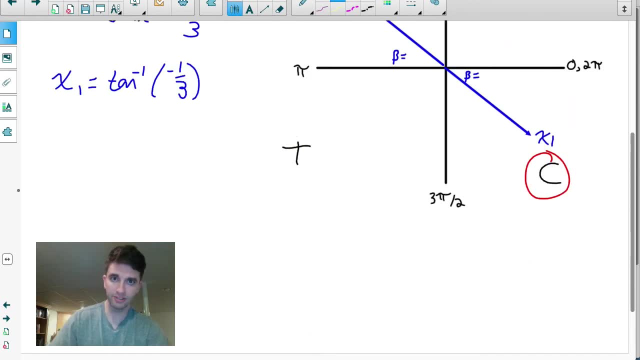 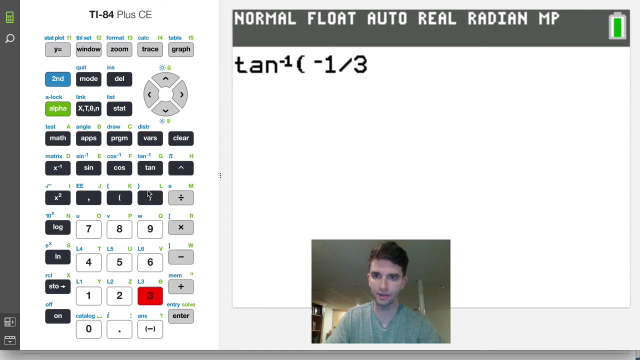 from the positive x-axis. Now there's going to be a little bit of a problem with us having that answer, but it is actually going to help us figure out the answer to the equation. So let's type this in on our calculator. So we're doing inverse tan of negative, a third and, like I said, the calculator is going. 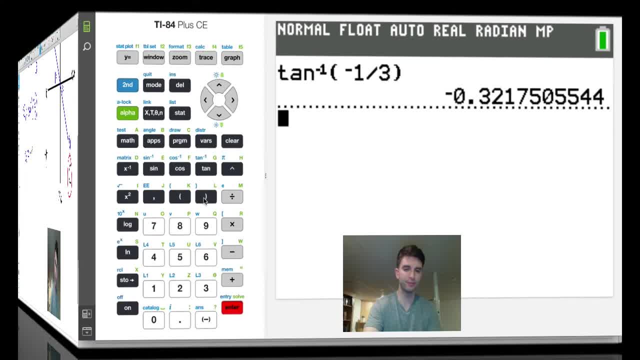 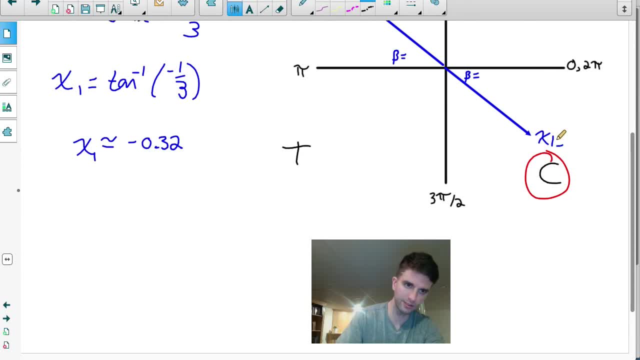 to actually give us a negative answer. It gives us negative .32 radians. So the calculator gave us an angle of negative 0.32.. So it said x1 is about negative 0.32.. There's a slight problem with this because this doesn't meet the criteria of the question. 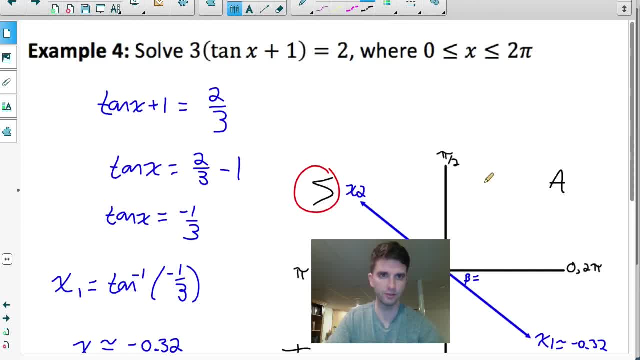 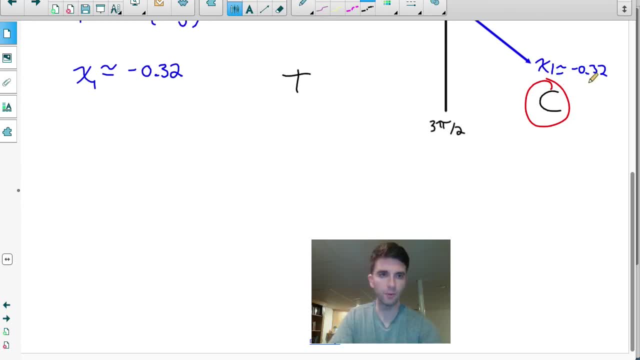 The question says: find all values for x that are between zero and two pi. Well, this is not between zero and two pi, So this is not a sufficient answer to our equation, But we can use it to help us actually figure out an acceptable answer. 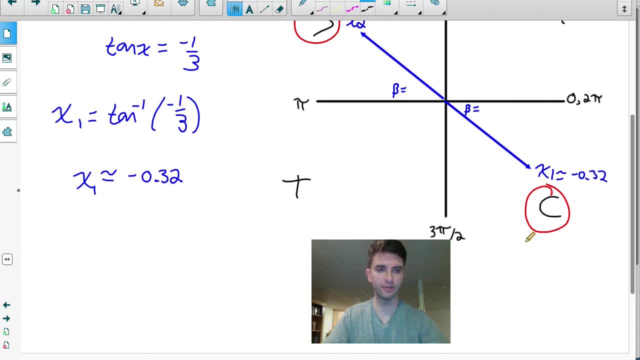 We're going to find an angle that is coterminal to negative .32.. What's a coterminal angle? It's an angle that has the same terminal arm as negative .32.. So how do we find a coterminal angle? 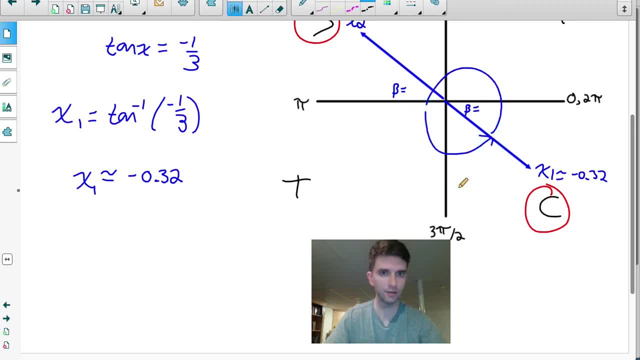 Well, we just add two pi. We add two pi to any angle. it brings us back to the exact same spot. It's a coterminal angle. So all I have to do to get a coterminal angle to negative .32, that is, between zero and two. 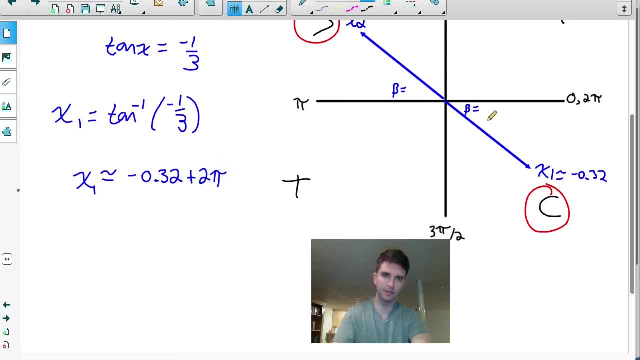 pi, just add two pi to it. If I'm here, just add two pi and you're right back to the same spot. So we do negative .32 plus two pi. we get a coterminal angle. So let's just add two pi to this angle. 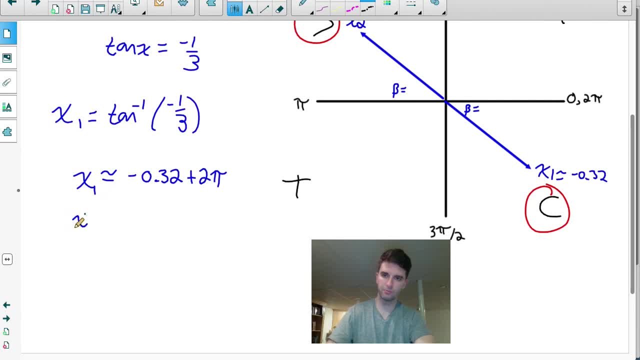 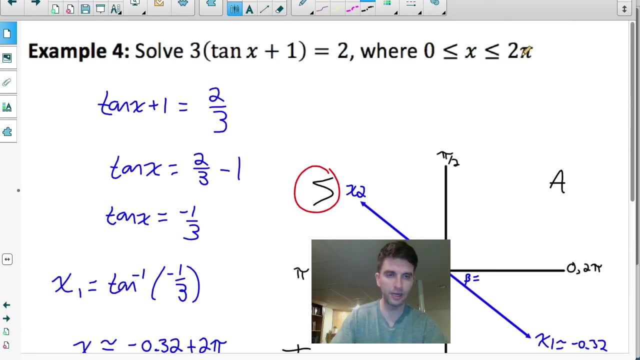 And we get 5.96.. So 5.96.. That is an acceptable answer to this equation. That is between zero and two pi. Two pi is about 6.28.. So we're between zero and 6.28.. 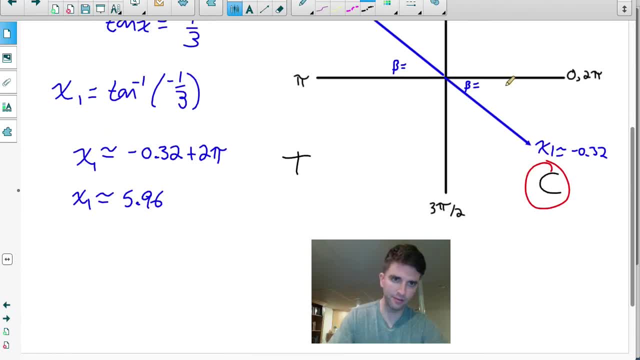 So that's an acceptable answer. Make sure you understand that if we went negative .32 radians, that means .32 that way, Or if we went 5.96 radians, that means 5.96 that way. They both land us in the exact same spot, so of course they have the same tan ratio. 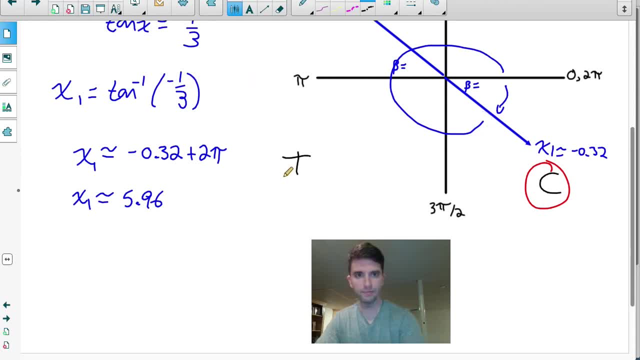 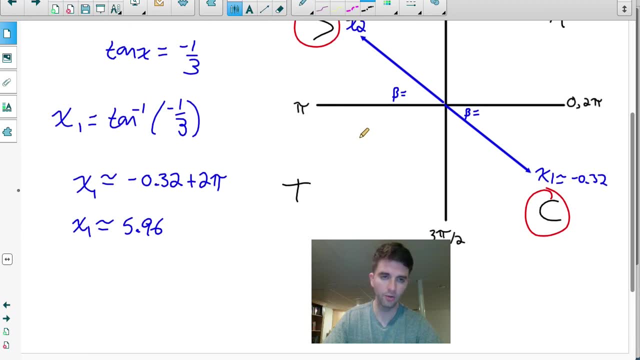 And they both have a tan ratio of negative a third, and that's what we want. So we have found one answer. How do we find the second answer? How do we find the answer that is in quadrant number two? Well, what we have to do is place whatever the reference angle for this one was into.